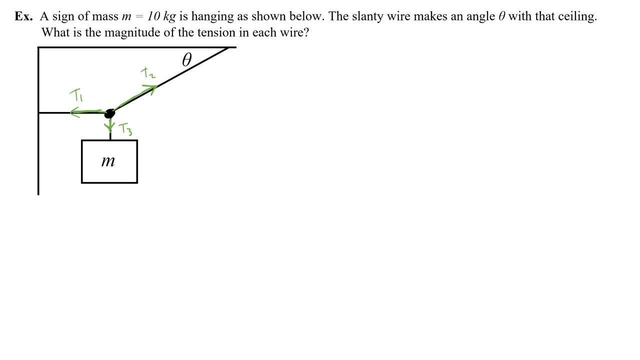 let's start with the easiest of these, and that is this T3.. So if there's a tension pulling down on that little knot, then there is a tension also pulling up, And those tensions are equal to each other because this thing is balanced, So the downward tension on the knot is equal. 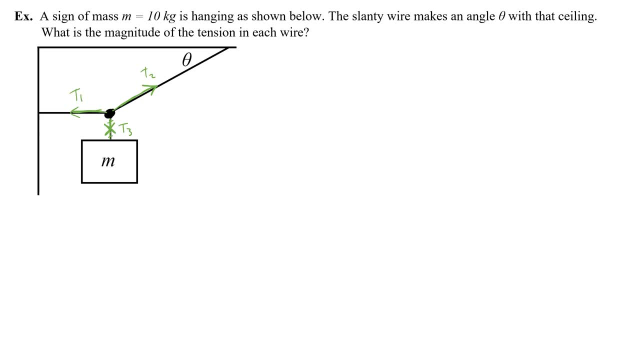 to the upward tension that's holding the mass up. Well, what would that be equal to? Well, there's going to be a weight force acting down, And so T3, downward tension, is just equal to mg. So there's the first thing, right. I know that T3,. 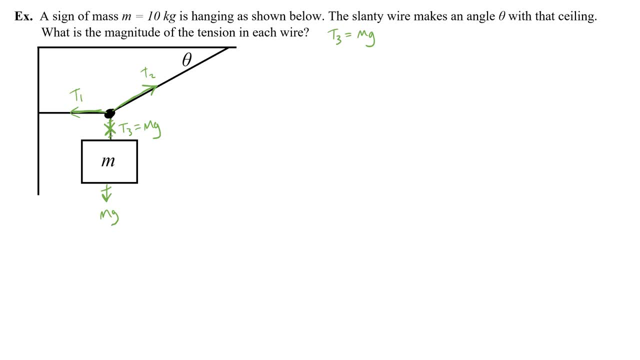 the tension down is equal to mg, which you know, using m is 10 kilograms and g is 10 meters. per second squared gives me 100 newtons. Okay, well, now let's move on to T1 and T2.. And also let's. 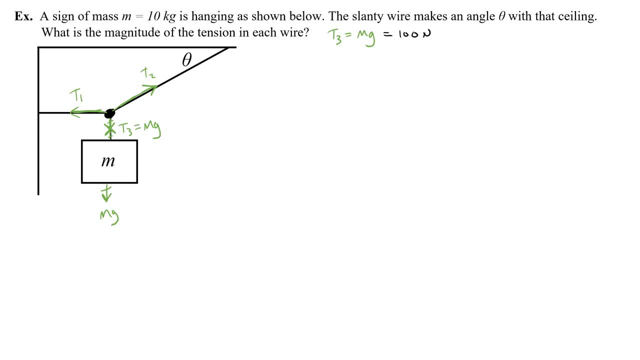 talk about the fact that sometimes this problem will be presented without that third wire hanging down. Sometimes it'll just look like this, Where you have the wire on either side of the object. Now, in this case, the problem looks the exact same. You got T, it'd be like T1, T2.. But instead of a T3,. 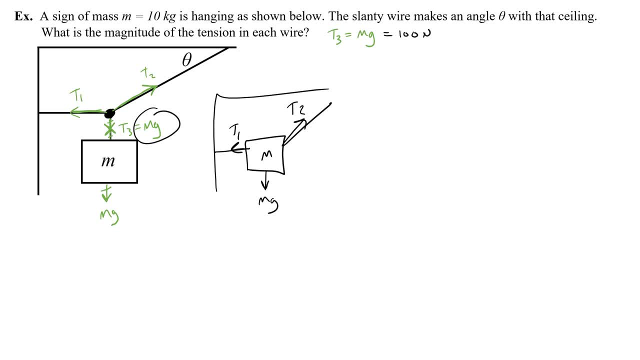 you just skip right to the fact that it's mg And in fact it sort of simplifies the problem if we approach it this way when we're looking at T1 and T2.. So let's draw a dot representing the knot where all those wires connect And let's draw sort of an enlarged 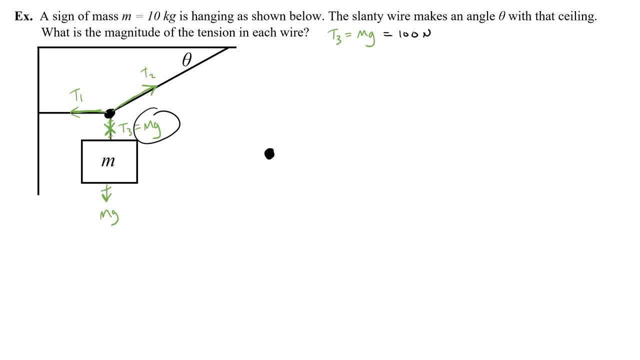 free-threaded, free-threaded, free-threaded, free-threaded, free-threaded, free-threaded, free-threaded diagram on that dot so that we can better represent what's going on. So the first thing I have is that tension T1, that's horizontal and to the left slanty tension T2.. And then 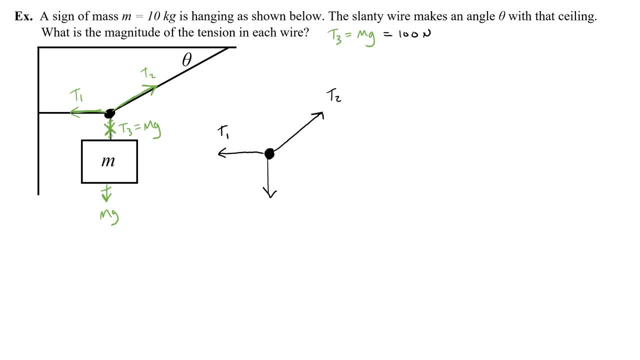 instead of saying T3 down, I'm just going to go ahead and say, mg, Okay, cool. So where do I go from here? Well, I know that I have to do something with this tension at an angle, And converting the tension into an X and a Y component is probably a good. 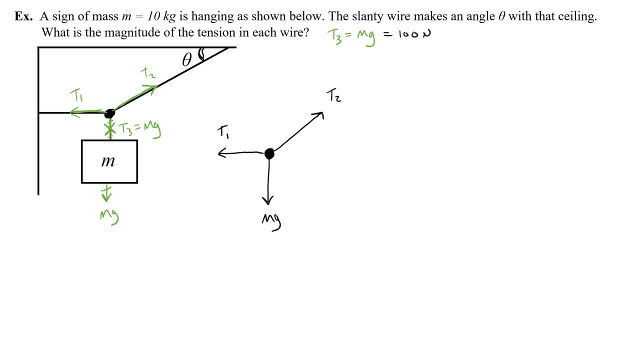 start Doing. that is a little complicated because my angle is up with the ceiling And whenever we do components of vectors we want the angle to be down by the dot, somewhere down by that actual dot. So here's what I do: I draw my little Zorro thing. 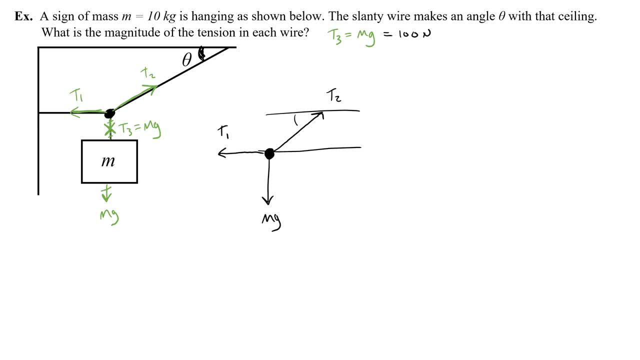 And I think if this is theta, then so is this. I forget what that is called in geometry, but it's something and it's true. So I know that my angle theta can go there And I'm going to use that angle to make an X and a Y component. Now, of course, 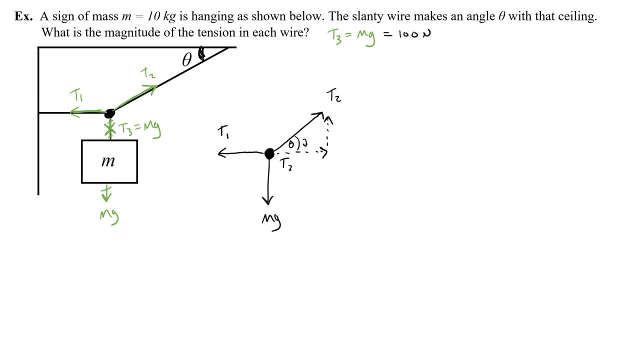 as long as this angle is adjacent, I'll use cosine, So T2 cosine theta for my X component and then opposite for the Y. So I would do T2 sine theta. Okay, classic X and Y components. Where do we go from here? Well, this problem is balanced right, We're in equilibrium. So 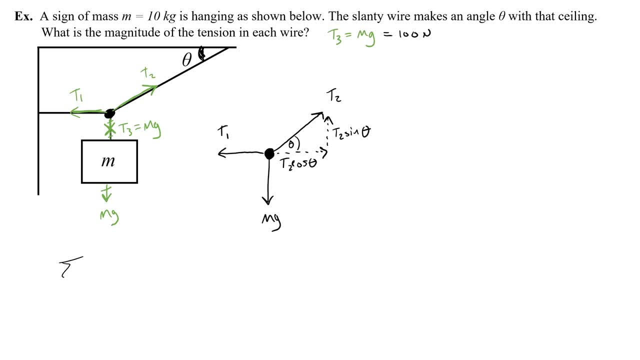 all the net forces on everything right, Sigma Fx and Sigma Fy, there's zero. Everything is balanced. So I'm going to do T2, cosine theta for my X component and then opposite for the Y. So that tells me that any forces at the point left are equal to the forces at the point right. 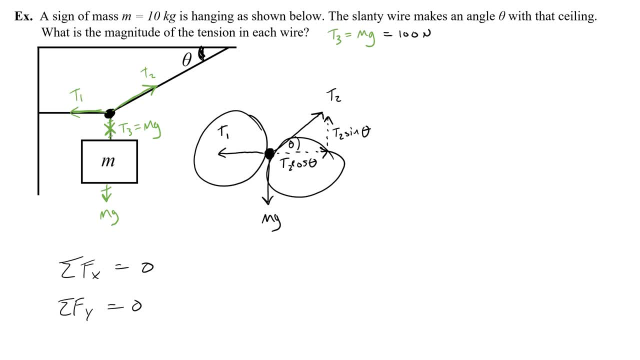 T1 is equal to T2 cosine theta And T2 sine theta is equal to MG. So let's do the X versus. I don't want to confuse you. T1 equals T2 cosine theta. Okay, so the left force equals. 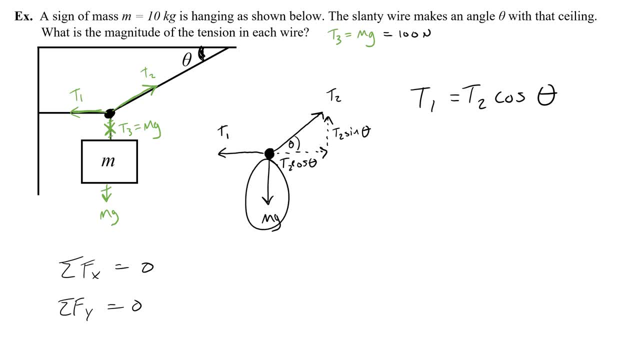 the right force. Then we look at the Y, MG and T2 sine theta. MG equals T2 sine theta. Okay, so now we have a system of equations and we want to find both T1 and T2, right, That's our. 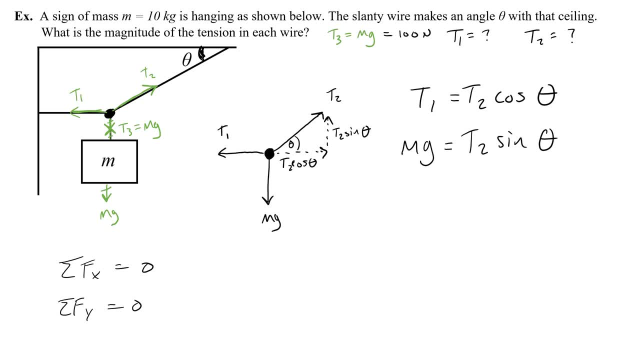 goal? We want to find the tension in all the wires. So how do we do that? Well, right away you probably would want to try and solve this system with substitution right. Just solve, maybe, this equation for T2 and then plug it in and thereby 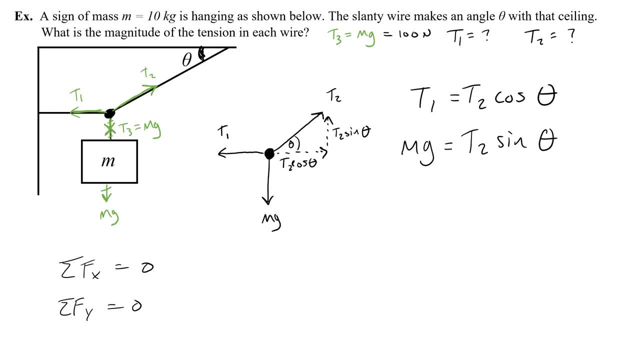 eliminate it, getting an equation for T1. And that's great, That would work well. But here's a new systems of equation trick that maybe you've learned before. maybe you haven't learned before. So with Atwood's machines and you know, two box problems, that sort of thing normally we make. 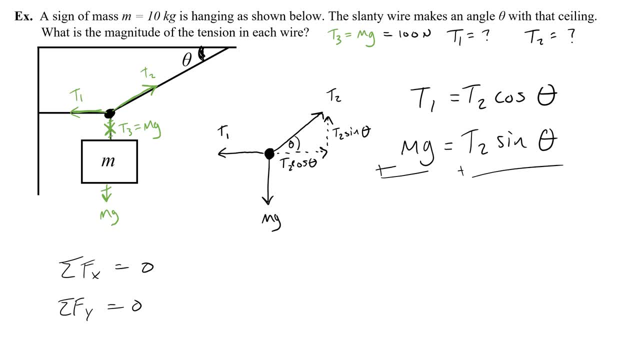 two equations or three equations, and then we add the left and the right sides because we're going to cancel something out. Well, you can add, subtract, multiply or divide both sides and still be able eliminate things. So in this problem, instead of adding the left sides together and the right sides together, 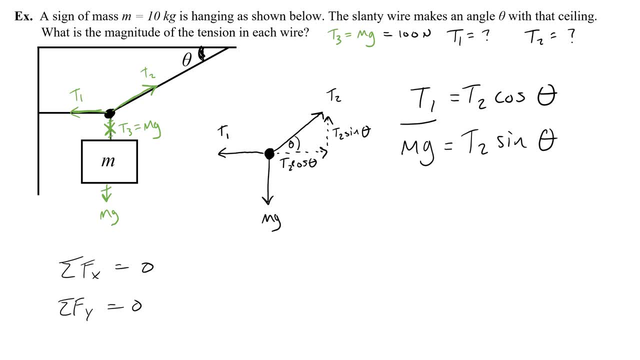 I'm going to divide left side by the left side and divide the right side by the right side. So doing this gives me T1 over MG, equals T2 cosine theta over T2 sine theta. Why would I do that? Because T2 cancels out And now I get T1 over mg, equals cosine theta over sine theta, which is cotangent. 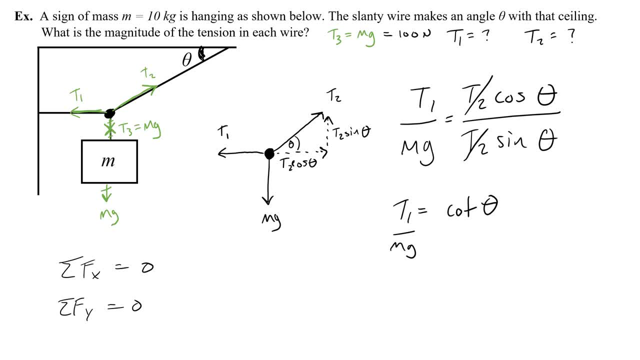 theta. in case you don't remember, You could leave it as cosine over sine. it's fine if you don't remember that cosine over sine is cotangent, And then to solve for T1, it's really easy, right? T1. 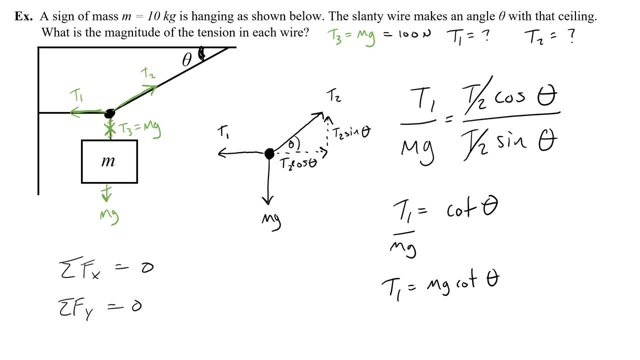 is just mg times cotangent of theta, because you multiply mg by to both sides. Okay, so let's get a number. The mass is 10 kilograms. g is 10 meters per second squared, so 100 newtons times cotangent. 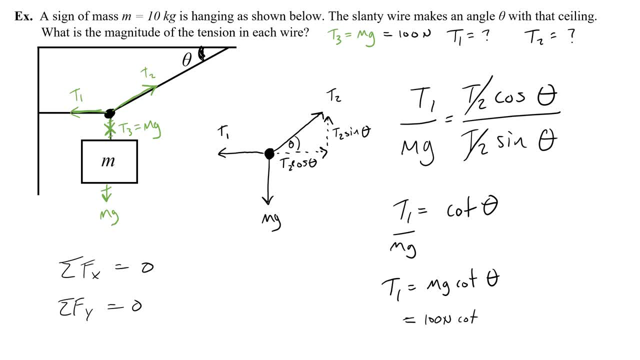 of. oh, you know what? they didn't give us an angle. Let's make up an angle right now, because this problem was supposed to have an angle. Theta equals 30 degrees. there it is cool, Okay, so let's use 30 degrees, Cotangent of 30 degrees. 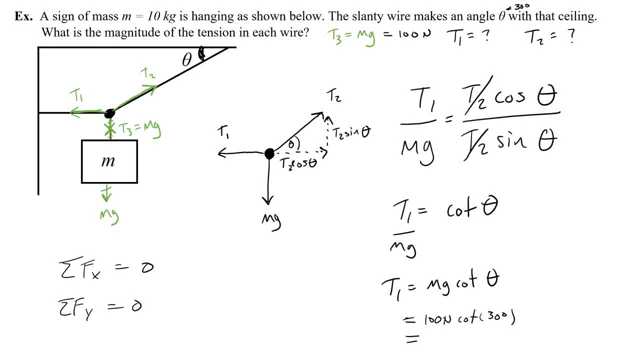 So 100, and make sure your calculator is in degree mode 100 cotangent, which is 1.7, so 100 times 1.73 is going to give us 173 newtons, It's like 173.2,. 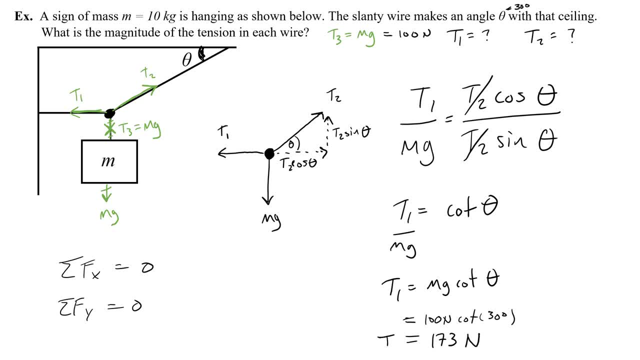 but let's just go ahead and call that 173 newtons. Okay, so that's T1.. 173 newtons- Now how do I find T2?? Well, I've got these two original equations. Let me get rid of. 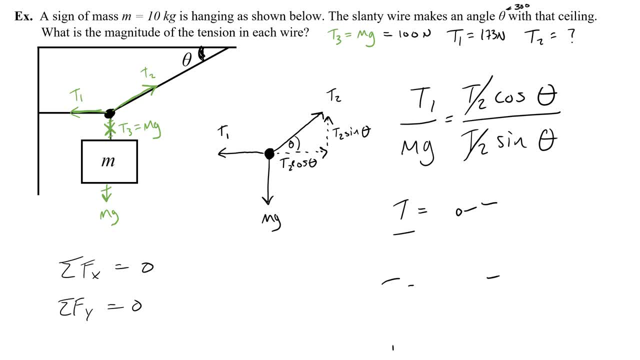 this work. right here I've got the two original equations that I wrote and now I can either plug T1 back into my T1 equals T2 cosine theta equation or I can just use this equation right here to solve for T2.. T2 is going to be equal to. 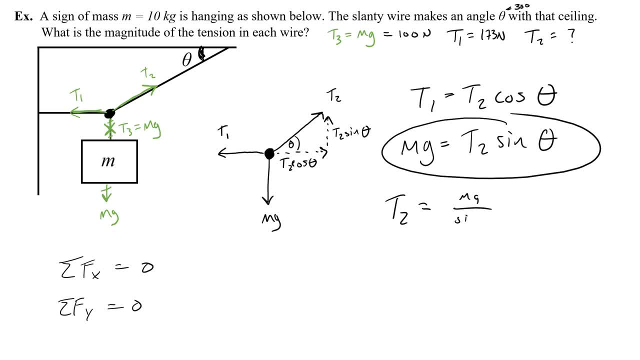 mg over sine theta. So this is going to give you 100 newtons over sine of 30 degrees, which sine of 30 is one-half. So 100 over one-half is like 100 times 2, so 200 newtons. Boom. We found the tension. 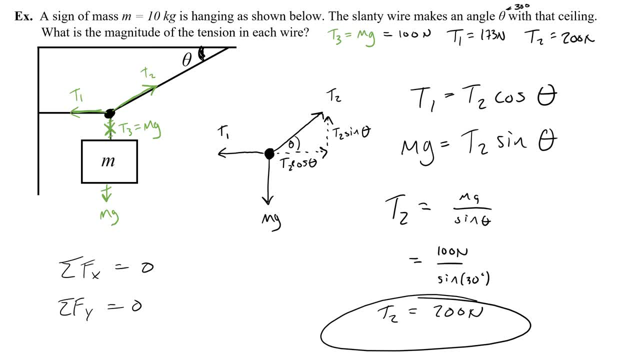 in the slanty wire? Okay, great, And you know. our general process is: we draw a free-body diagram, convert angled forces into components, then we write equations. If they're not accelerating, we don't set them equal to ma. 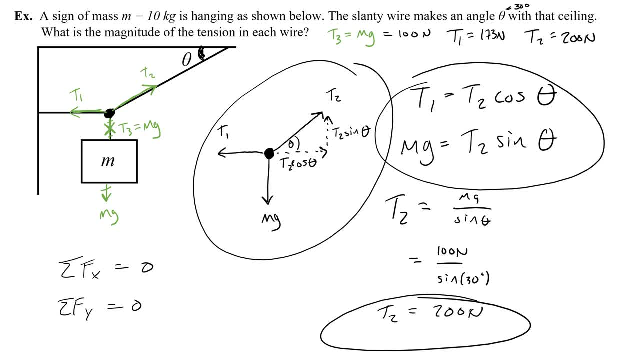 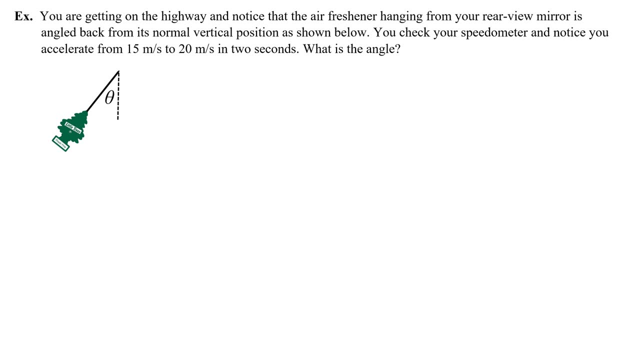 We set them equal to each other and then solve using some sort of clever trick. Substitution always works if substitution is the thing that you see as the quick and immediate solution. So now let's deal with a problem where there is a complicated tension and the forces are not. 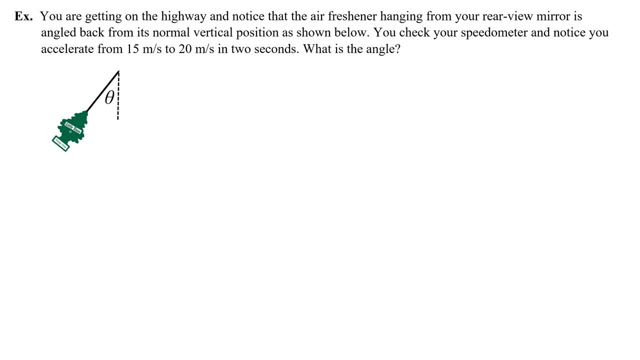 coming in, So there is an acceleration happening. This is a really fun problem. You are getting on the highway and notice that the air freshener hanging from your rear view mirror is angled back from its normal vertical position, as shown below. You check your speedometer and 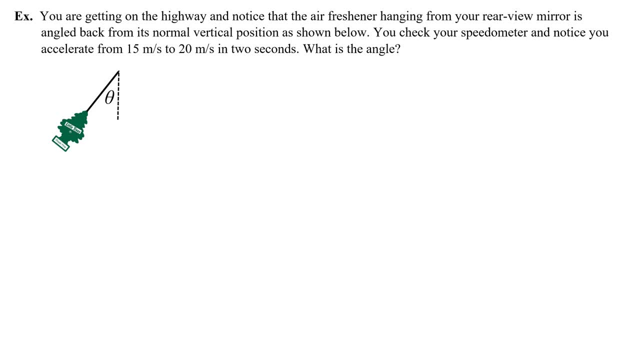 notice you accelerate from 15 meters a second to 20 meters a second in two seconds. Then you think, because you're zoning out and you're really smart, what is the angle? So what is the angle? well, let's, let's stop and deal with this first. this is an obvious 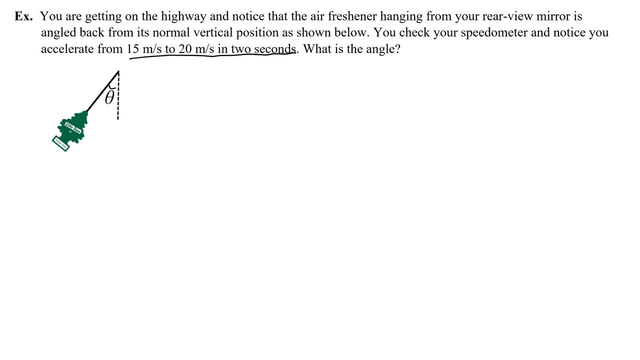 indication that there is an acceleration of the problem. right, because it says you accelerate. then it gives you information that you can use to find that acceleration. so let's find that acceleration right. V naught is 15, V is 20 and they give you a time of 2 seconds. how do you find the acceleration from? 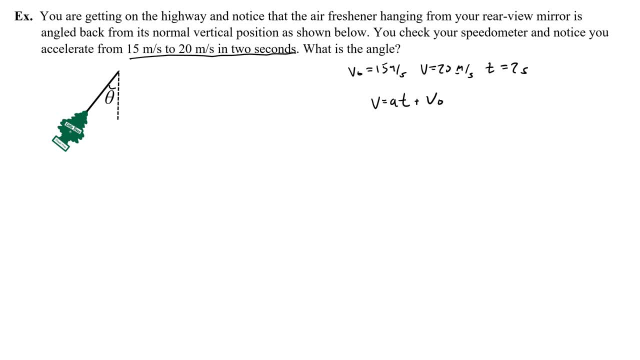 that well, you can take your motion equation that you're really comfortable using, or you can just use the fact that acceleration is change in velocity over a change in time. they're the same equation, just rewritten. so what's the change of velocity? you go from 15 to 20, so positive 5 in 2 seconds. so you divide. 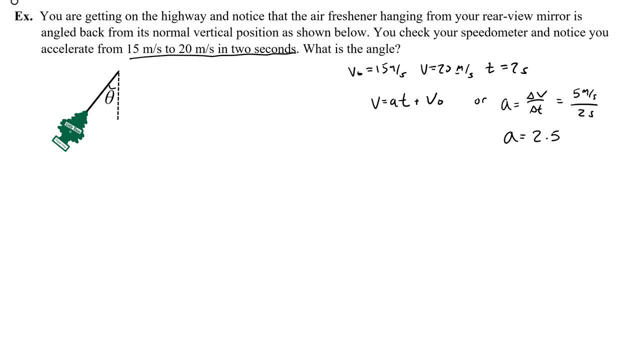 that by 2 and we get the acceleration is half of 5, or 2.5 meters per second, squared. ok, I'm going to get rid of this work, just so that we have some space to it to work. ok, so the acceleration is 2.5 meters per second and it's important to note that. 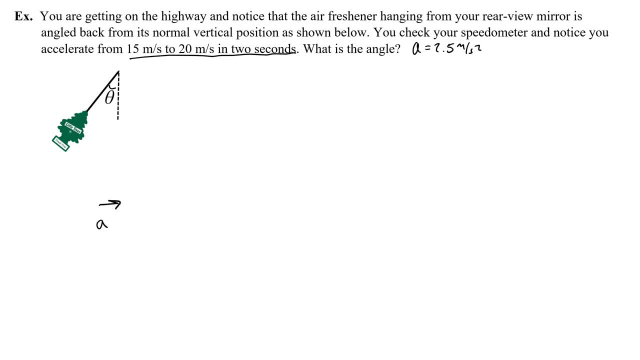 the acceleration is, we're assuming- horizontal. even there might be like a slight inclination if you get on the highway. let's just make this problem easy and assume your car is driving on the road and it's going, you know, to the right. there's a terrible car. I don't even know what that. 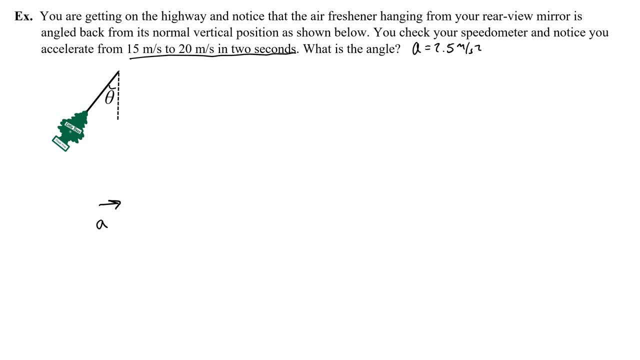 is ok. so, anyway, what do we do with this problem? well, we're going to draw a free body diagram for the air freshener and I'm going to draw this off to the right so that we have more room to work. so this dot represents the air freshener. 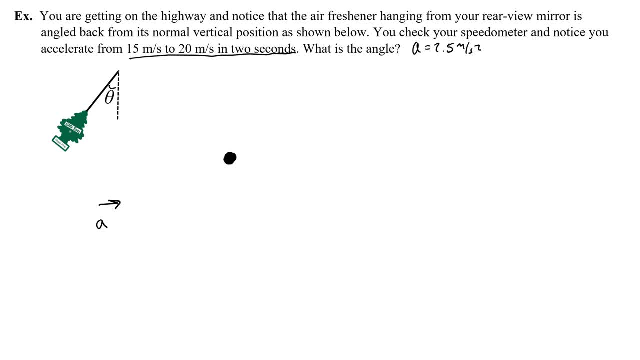 ok, and to figure out what that angle is, we're going to need to draw the force. there's a tension, right, your, your little trees, air fresheners hanging on by a string, so there's tension in that string T. and then there's this angle here, theta, ok. so this problem, first of all, we need 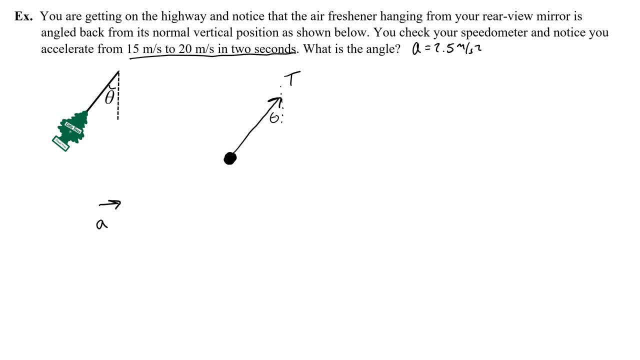 to deal with the angle. now. it's going to be a little bit different from the last problem, because now, instead of having an angle with the ceiling, we have an angle with respect to the vertical. so when I do my little Zorro trick tonight to make a Z, then my theta goes to the right. so I'm going to draw a free body diagram. 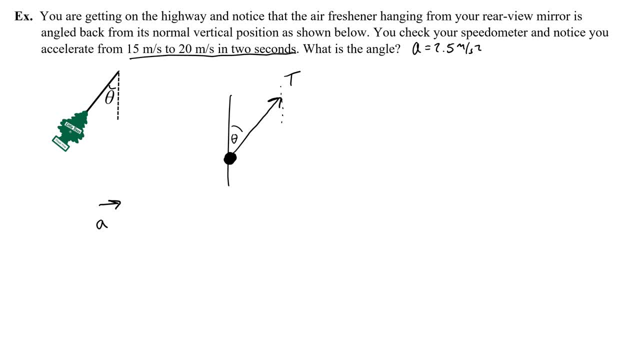 right here it's going to be a little bit different. I'm going to see if I can understand how this works. that you know, I have a little bit of tension between this and this node, which is actually where we had on before, so I need to find where the tension goes right. so, as for right, we're going to do this. one twenty seven D, everw остann it over there, so it's going to be a little bit wrong. so in the other side, right, we're going to add minus. I will add that here, and this one of those bucking up details attribute is a little bit. 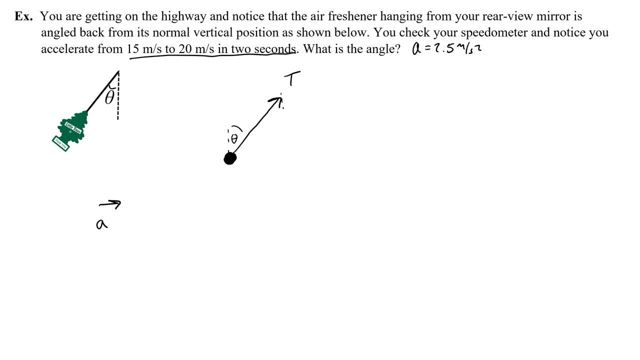 different from the last one. so, as a result that I'm going to draw this possible, in this case, I'm going to add this antagonist for the second time where I will have division, and so I'm going to draw at least two excerpts from the get. basically, this is going to work until I find out when. 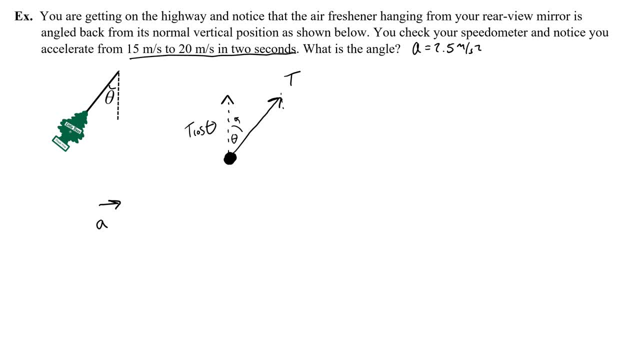 I'm going to construct what stay at least one of those decentralization cosine theta. so t cosine theta is now up, and then my x component, which goes to the left, is opposite of theta. so this would be a t sine theta force. okay, so that's the first thing, that's. 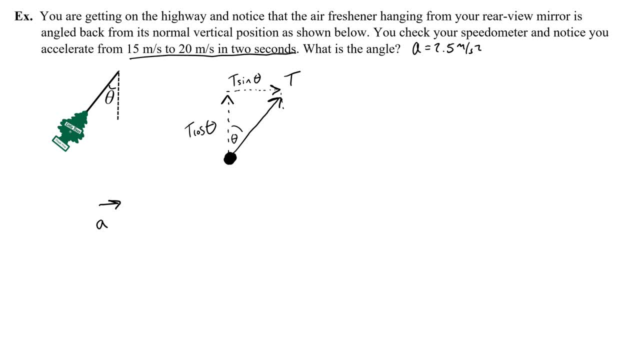 different. what else? are there any other forces acting on this object, like a force that's always acting on objects near the surface of the earth in a downward direction, with a really interesting factor that stays the same? yeah, there's a weight force. right, this thing has some weight, that's. 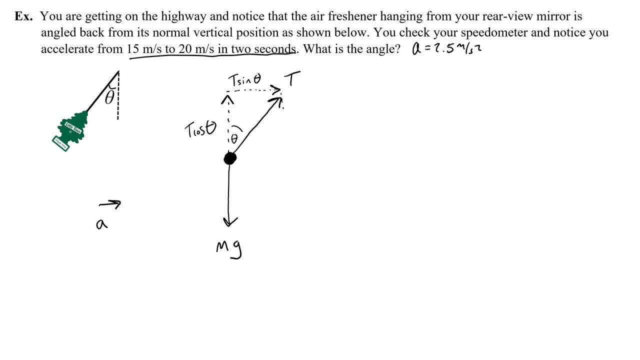 going to be equal to mg. now notice, we are not told what the mass of this air freshener is, and that's not a mistake that i made, like in the last problem, when i forgot to give you an angle. that's intentional. somehow in this problem we are going to get rid of that. that mg. 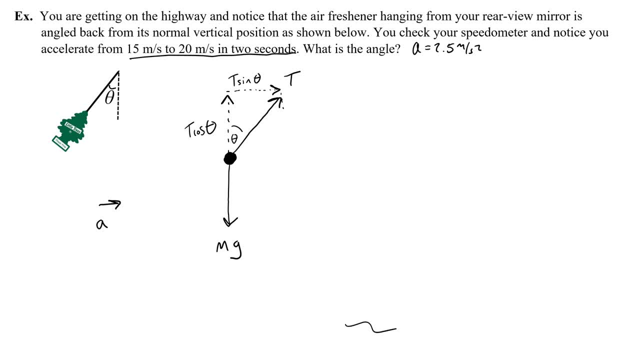 and we're going to get rid of that mg, and we're going to get rid of that mg and we're going to get rid of that mg, and doing so is a little tricky, so let's let's start by thinking about forces that are balanced. this thing is accelerating to the right. it's not accelerating. 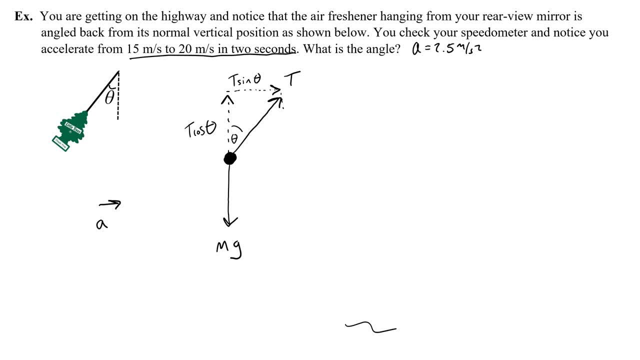 up or down, which means that my up and down forces are equal to each other, or t cosine theta is equal to mg. so t cosine theta equals mg. okay, well, so what about t sine theta? it's acting to the right. there's no force acting to the left for it to be balanced. 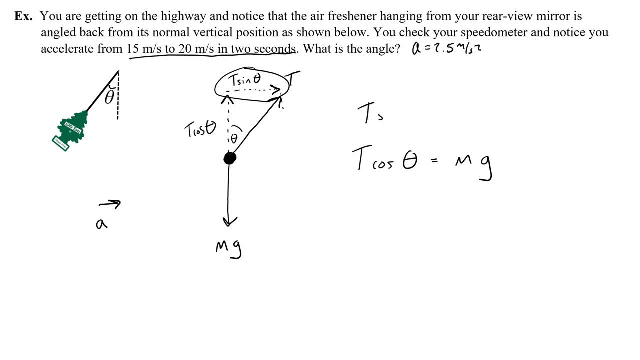 by how do i know what to set it? equal to well, if there's no force acting against it, then that means that we have unbalanced force. so if t sine theta is unbalanced, that means it's the net force, and the net force is always equal to mass times acceleration. so t sine theta is equal to mg. 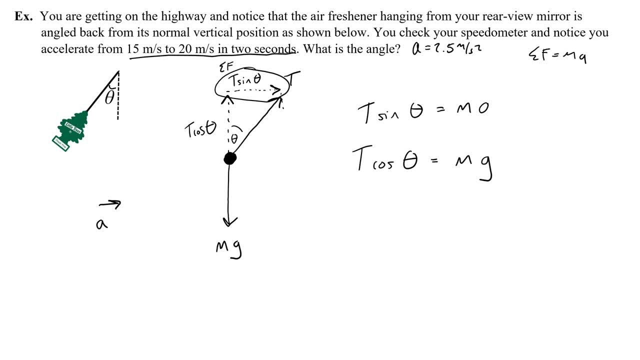 and t is equal to the mass of the little trees times acceleration. why is important? is it sorry? why is that important? why did i do that? well, now, if we apply our little divide the left sides and divide the right sides trick, so then t cancel out and m cancels. 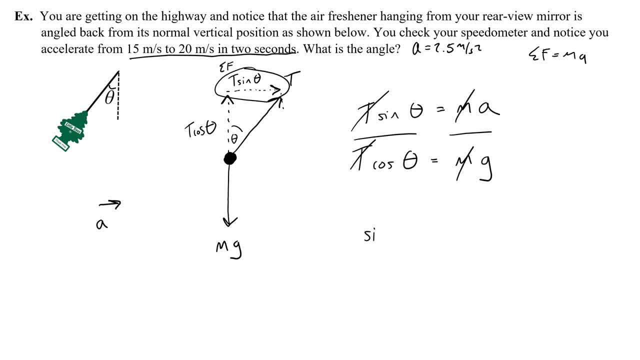 out. that's crazy. what i'm left with is sine theta over cosine. theta equals the acceleration, because i a. 0 for the first, tenemos la嫌nis. 0 for the first, tenemos la excelunga. 0 for the first, tenemos la excelunga. 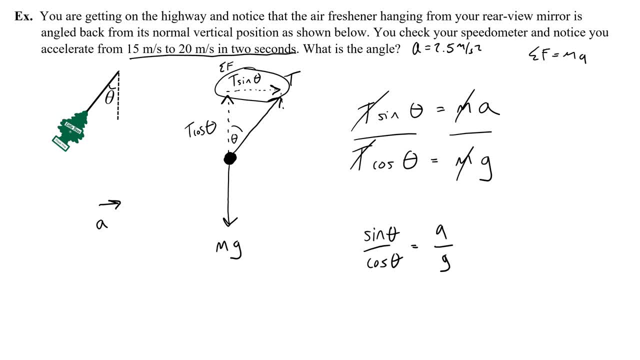 the car over g, the acceleration due to gravity and, of course, sine over cosine, theta is tangent theta. this is like this is wild. so so, first of all, um, a couple of things. if i could rewrite this to say: uh, acceleration equals g, tangent theta. and what that would mean is that if, if i had, 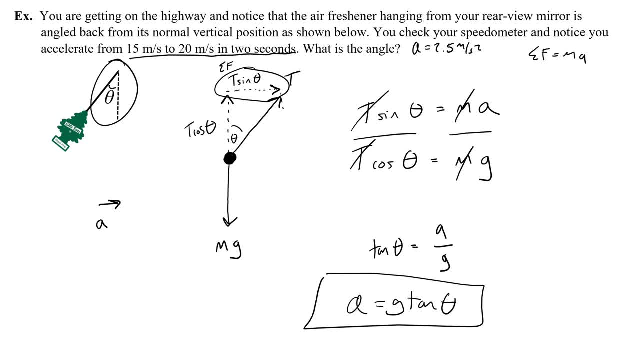 some way of measuring theta um in my car. like if you put, like if you hung a protractor from the rear view mirror of your car, then, based on what the angle that the string makes with that protractor, you could calculate your exact acceleration of from your car. 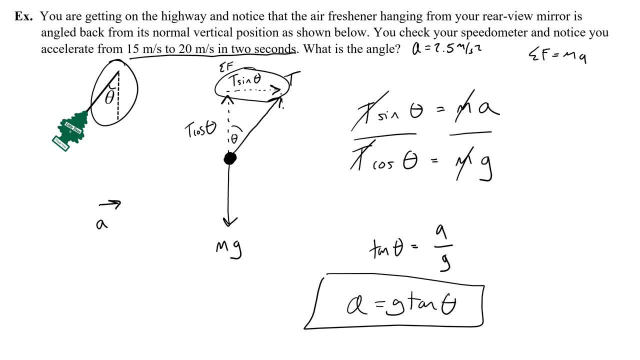 without ever having to get a stopwatch or a meter stick or anything like that. so, um, physicists use this. it's a very special apparatus. it's called an accelerometer. an accelerometer is a way of measuring acceleration without actually needing to take any any time values. you just have to look at what is it, what angle is made? 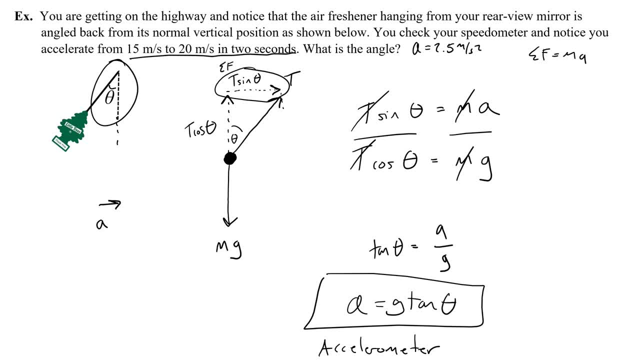 with a vertical line like that. and then also, what planet are you on? because if you're on the moon, then your air freshener is going to have a a very different angle than it would be on the earth. okay, but so that's besides the point. we're not looking for the acceleration here, although if we need.